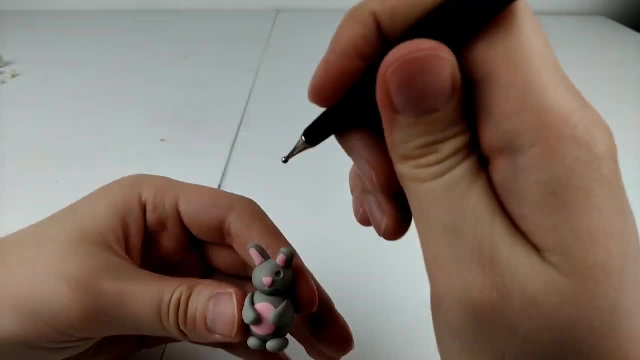 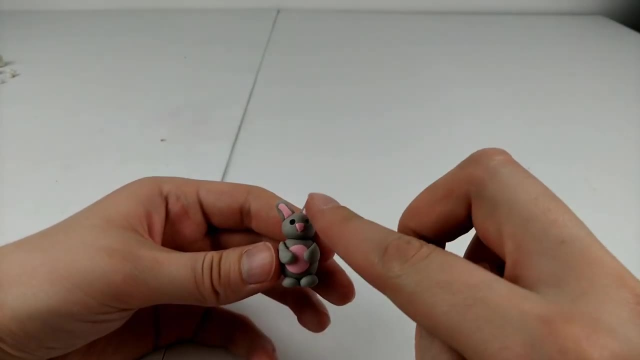 Now I'm just going to make some indents for the eyes. You could use a sculpting tool or even a bobby pin, And then we'll roll out small balls of black clay to put them. I actually decided I didn't like how the nose 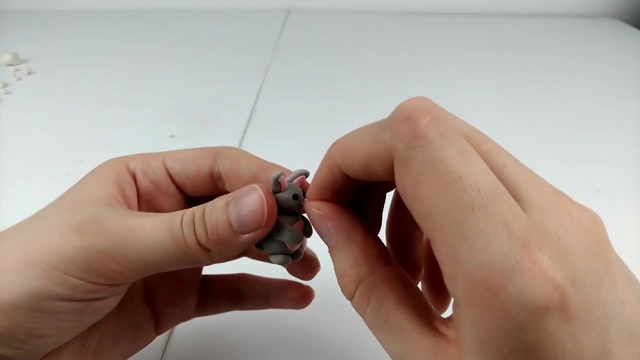 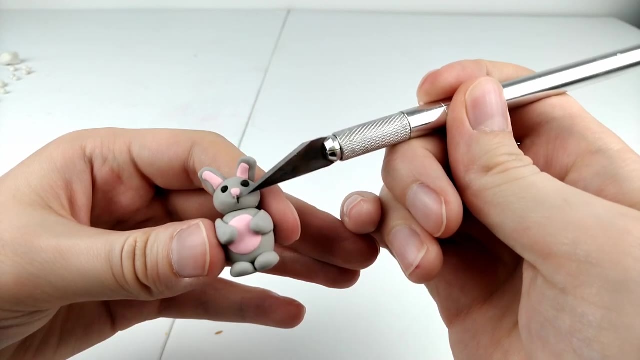 looks. so I just took it off and replaced it with a slightly smaller one. Not a big difference, but apparently it mattered to me. I also rolled out very, very thin strips of black clay for the mouth. This part was pretty tricky. 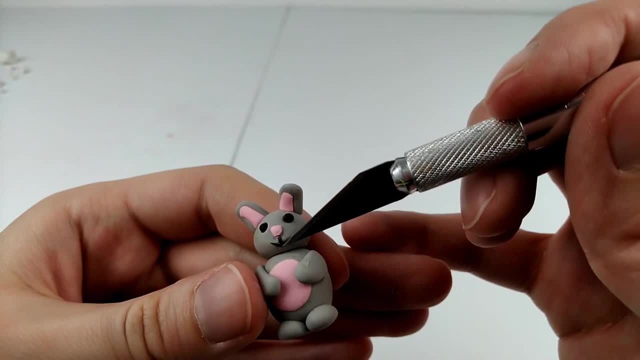 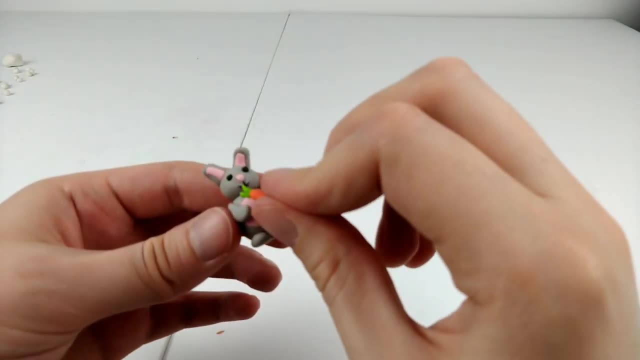 but I find it easier rolling it on a piece of paper, as it adds more friction and it doesn't stick so easily. And the bunny's arms just looked empty, so I thought I'd add in a carrot too, And after baking, our little bunny is complete. 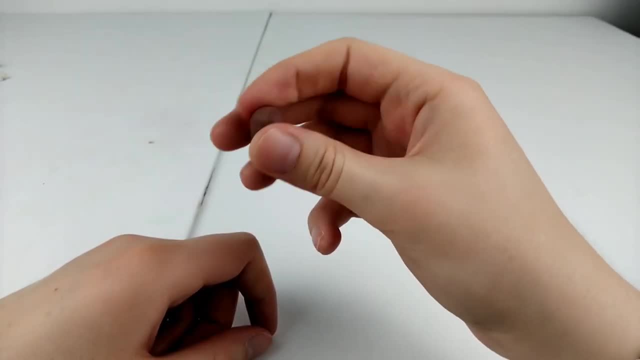 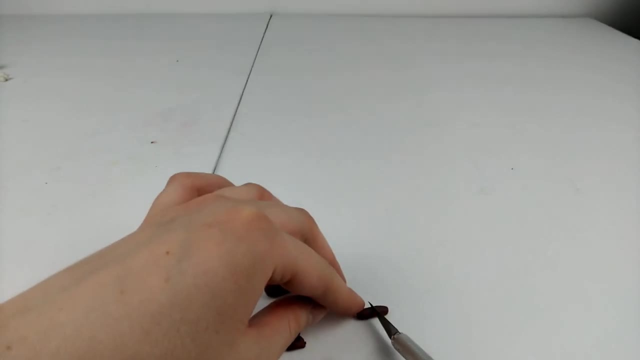 And next is the sheep. So let's just take a ball of brown clay and roll it out into a fat log, And we're going to take smaller balls of clay and roll them into littler logs for the legs. Littler, Is that a word? 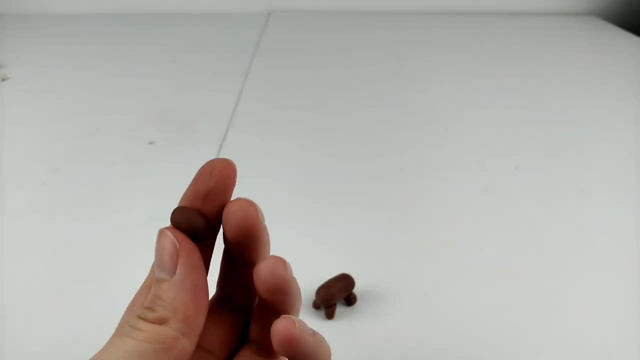 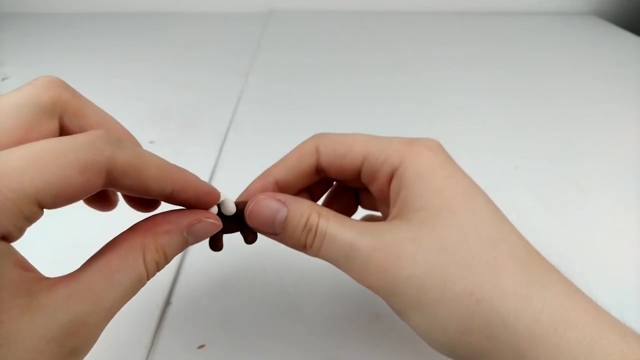 And for the head? we're just going to take another ball of clay and slightly roll it between our fingers to give it an elongated face. And now comes the fun part. We're going to take a bunch of little white balls of clay and we're just going to stick them all over the sheep. 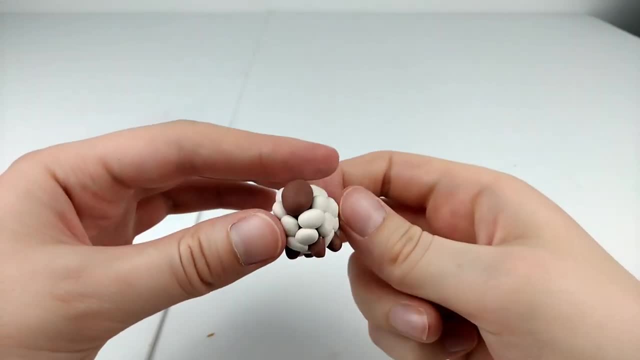 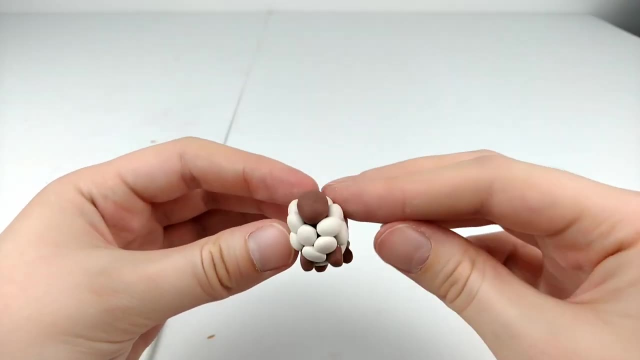 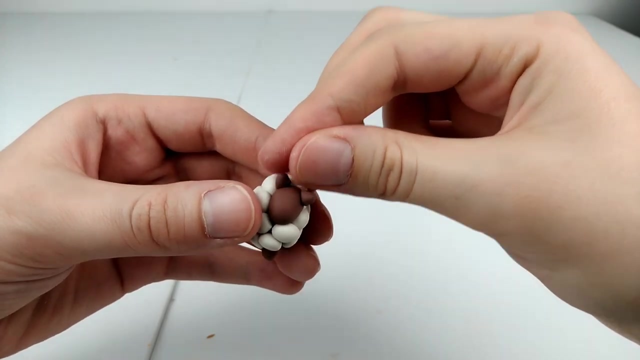 And you're probably going to need a lot more than you originally thought. And last one: Now, let's just give our little guy some ears. Now, let's just give our little guy some ears. Just using a log, cut in half And once again, just make two indents on the face and fill those with little black balls of clay for the eyes. 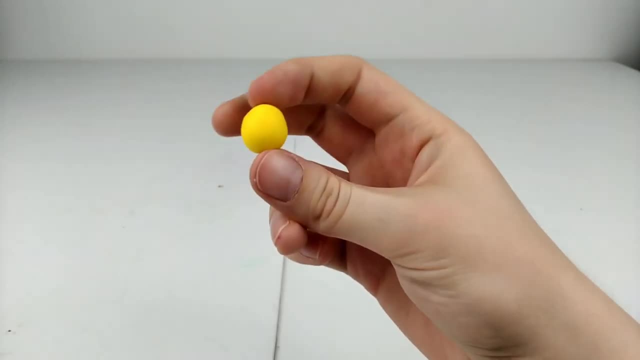 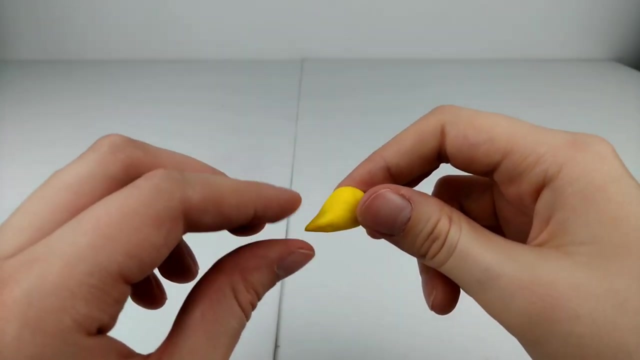 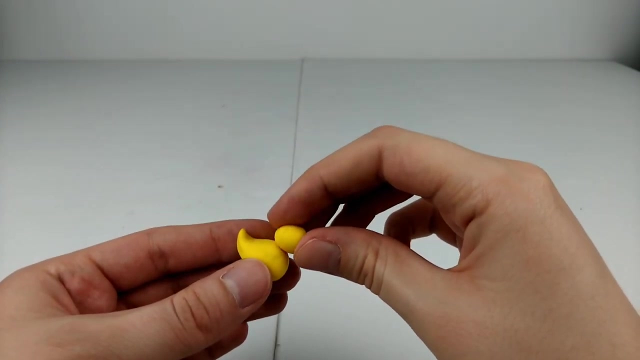 And your sheep is done. Moving on to the duck, let's start with a ball of yellow clay and pinching the end into sort of a teardrop shape and flip it up at the top. Once that's done, take a smaller ball of yellow clay and put that on top as the head. 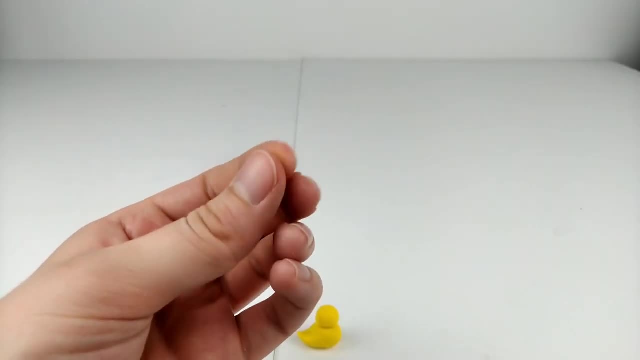 Once that's done, take a smaller ball of yellow clay and put that on top as the head. And once that's done, take a smaller ball of yellow clay and put that on top as the head. And once that's done, take a smaller ball of yellow clay and put that on top as the head. 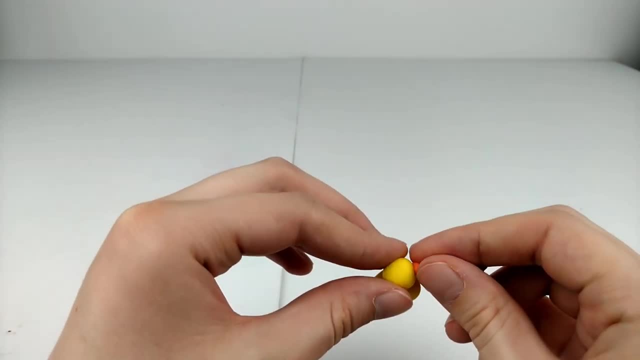 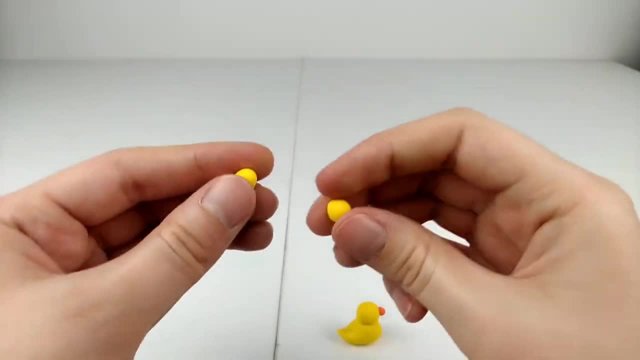 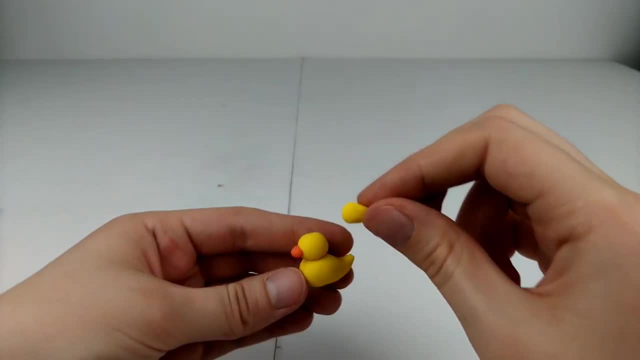 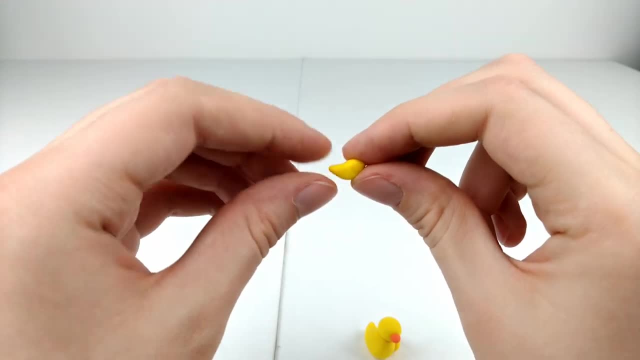 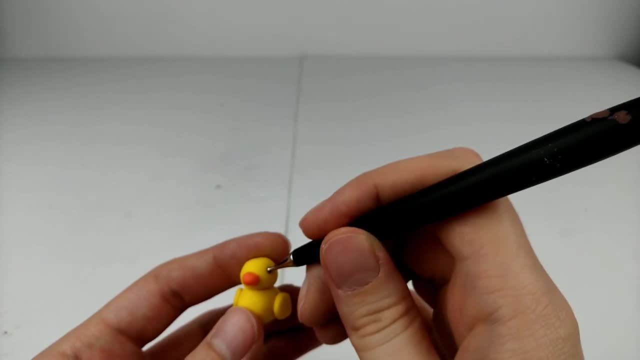 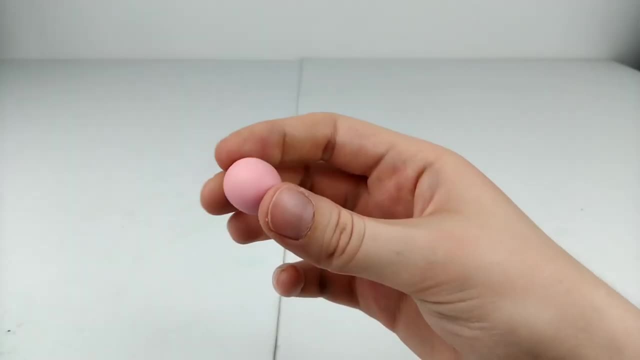 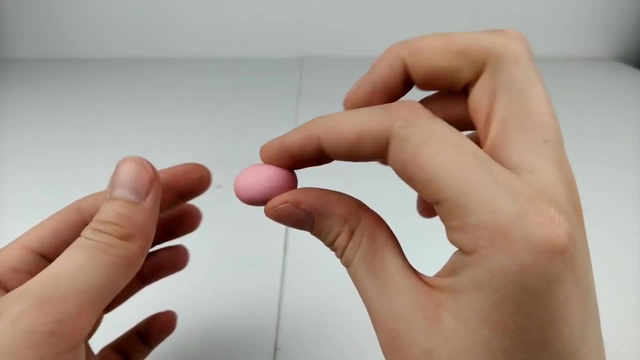 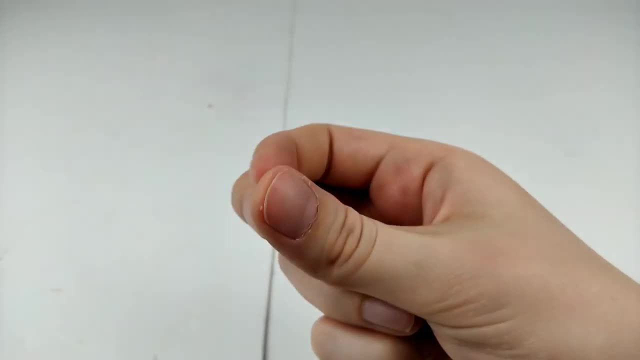 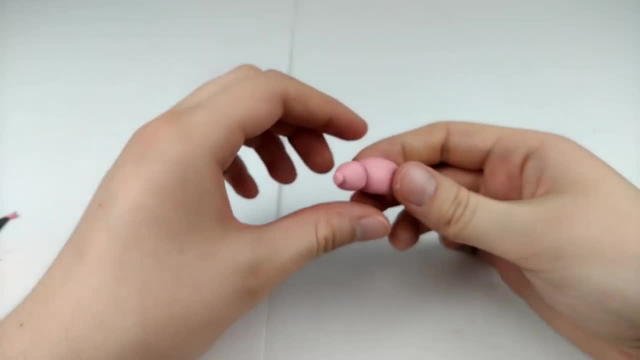 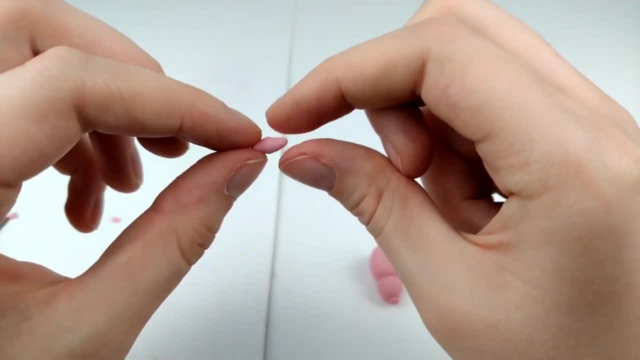 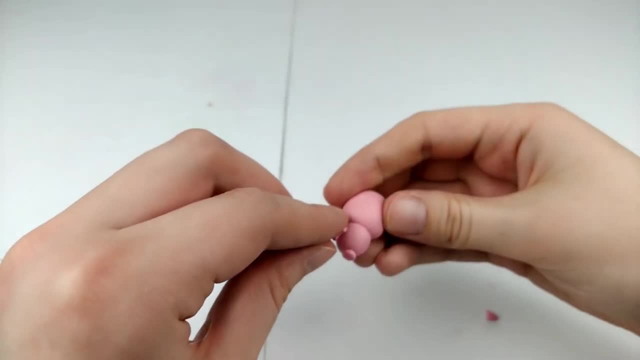 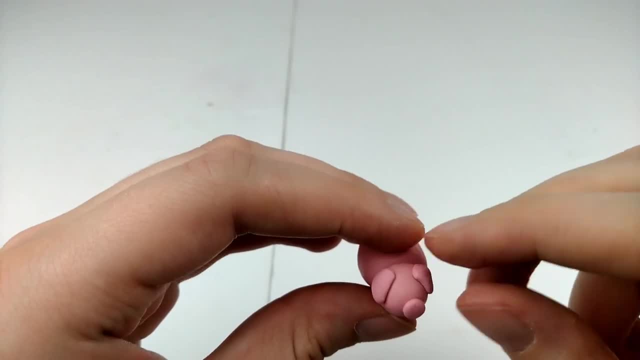 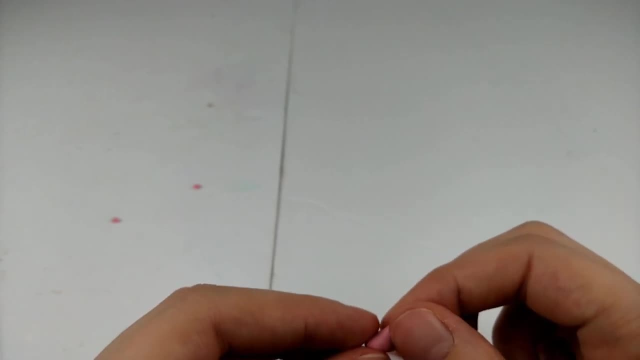 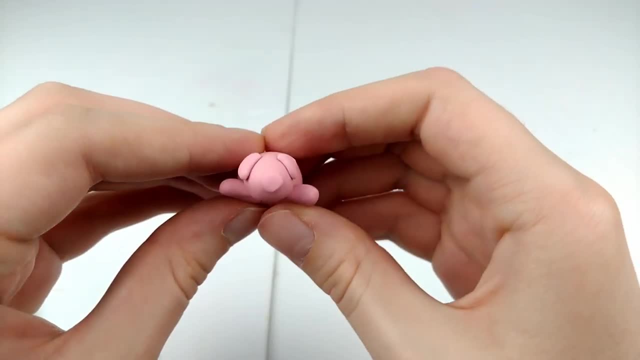 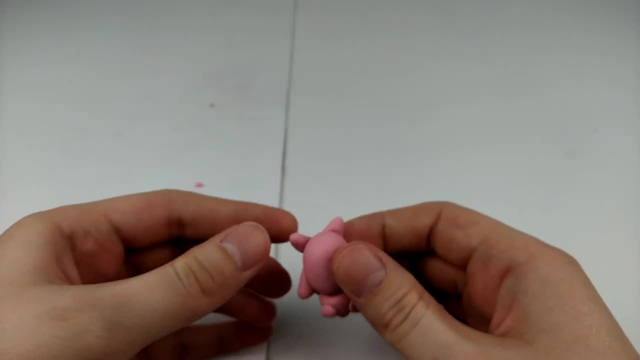 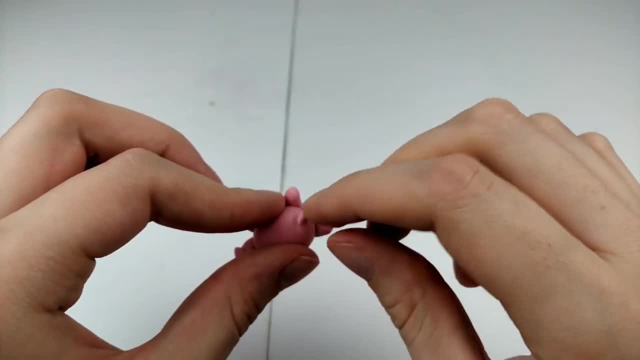 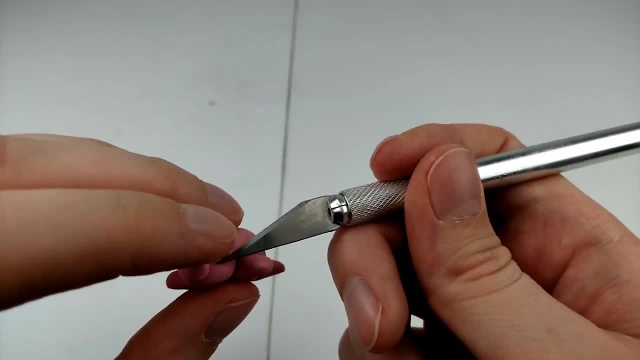 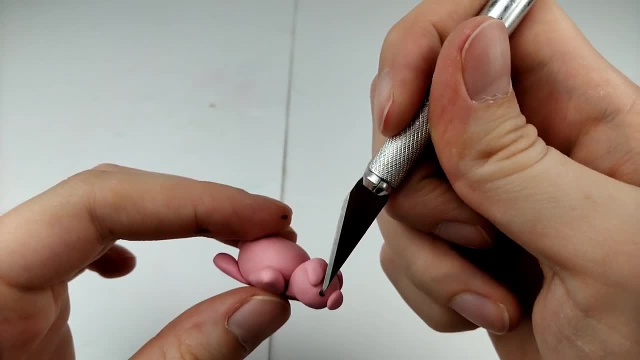 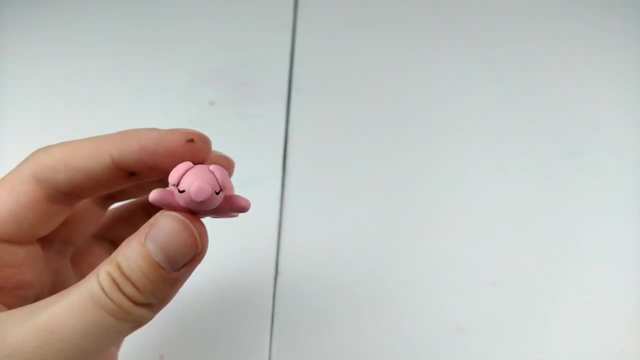 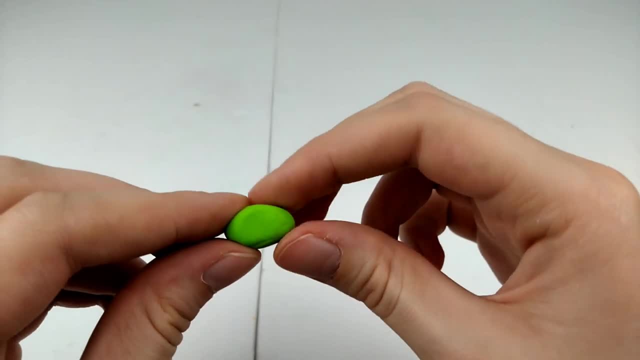 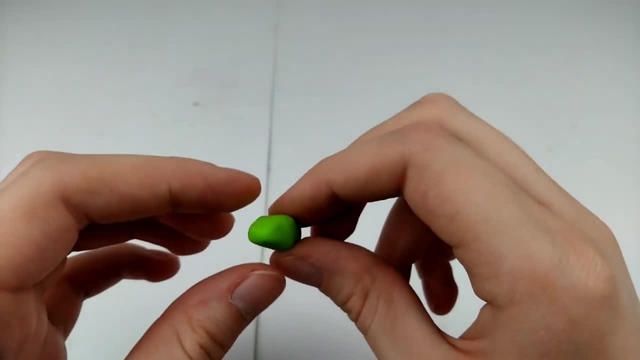 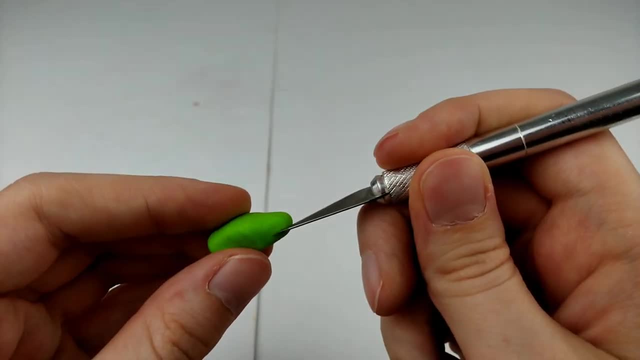 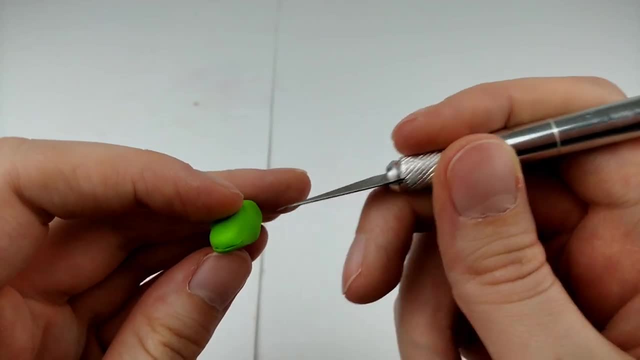 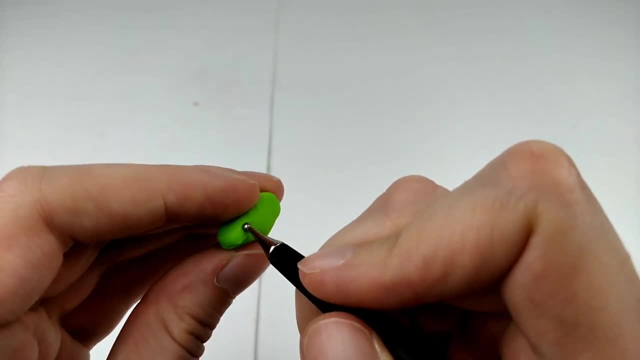 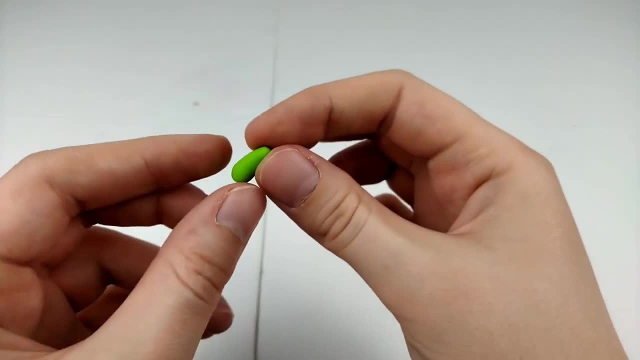 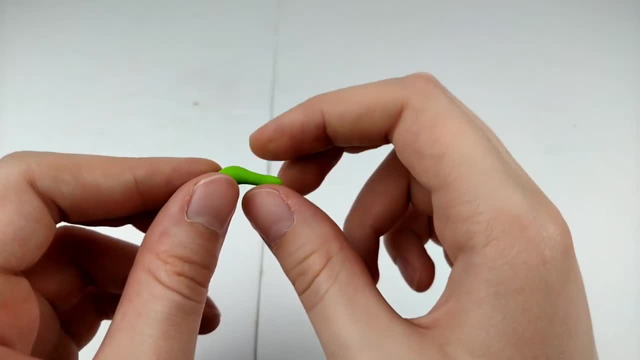 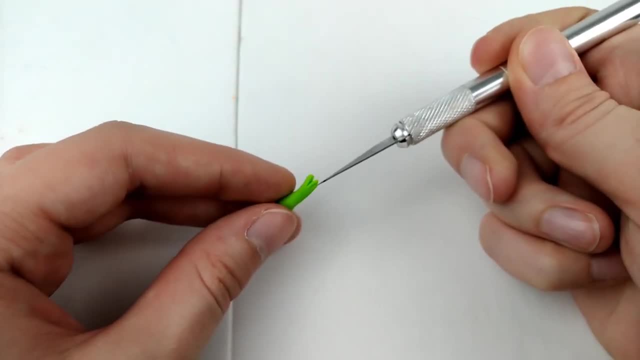 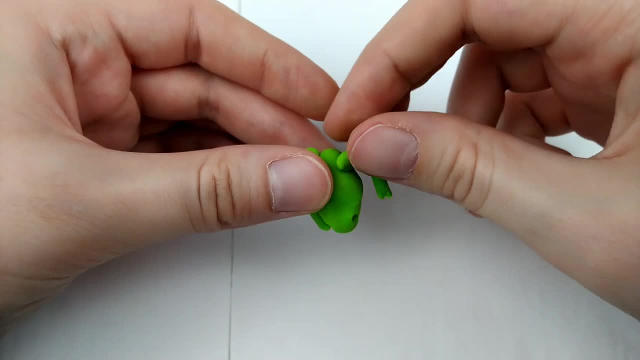 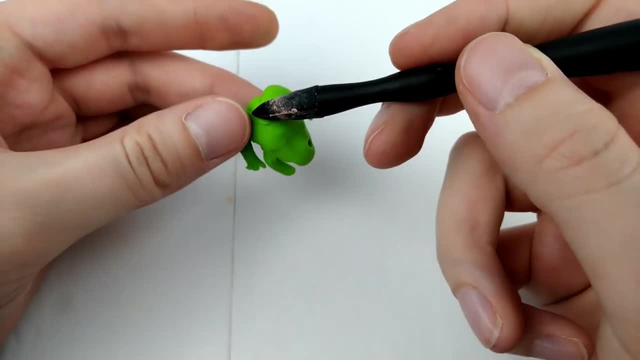 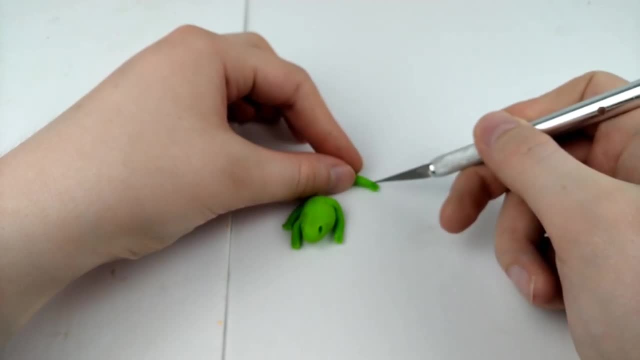 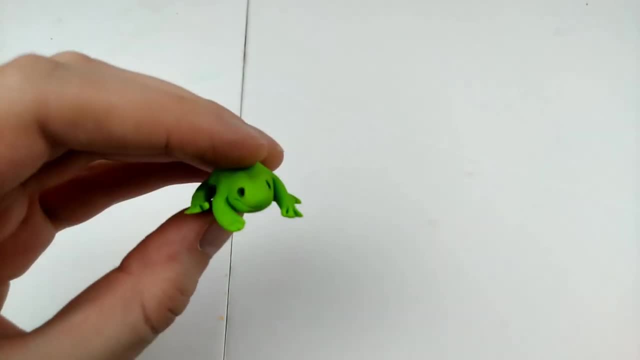